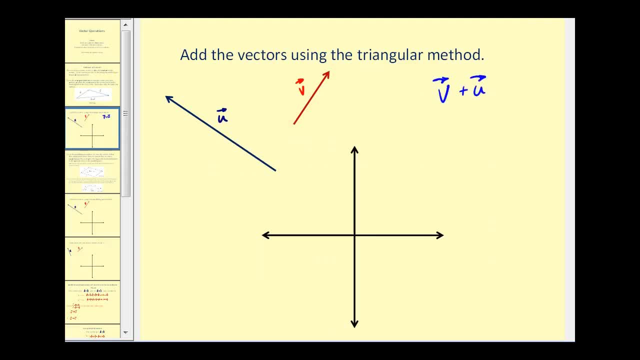 the sum of vector V and U. We'll go ahead and graph vector V as a position vector. Now we'll graph vector U, starting at the terminal point of vector V. So the resultant vector, or the sum of these vectors, would be this vector. 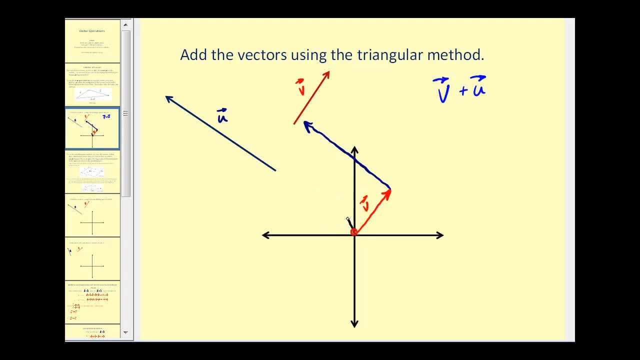 that has its initial point at the origin and its terminal point at the terminal point of vector U, And this is the tail-to-tip or triangular method. If we wanted to know the magnitude of the resultant vector, we could measure this with a ruler, and we could also find the direction angle with a protractor. 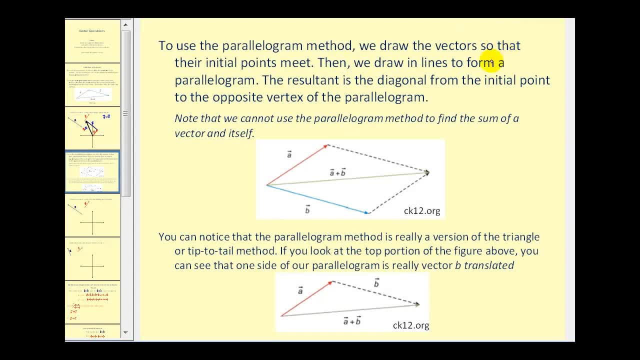 To use the parallelogram method. we draw the vectors so that their initial points meet, Then we draw in lines to form a parallelogram and the resultant is the diagonal from the initial point to the opposite vertex of the parallelogram. So here's vector A plus vector. 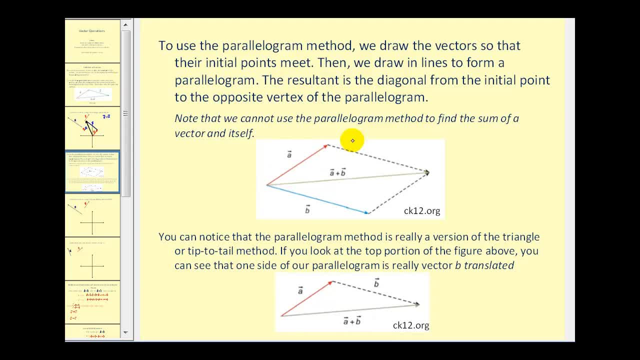 B. Notice they share the same initial point. The dashed vectors would construct the parallelogram and the diagonal is the resultant or the sum of those two vectors. You can notice that the parallelogram method is really a version of the triangular or tip-to-tail method. 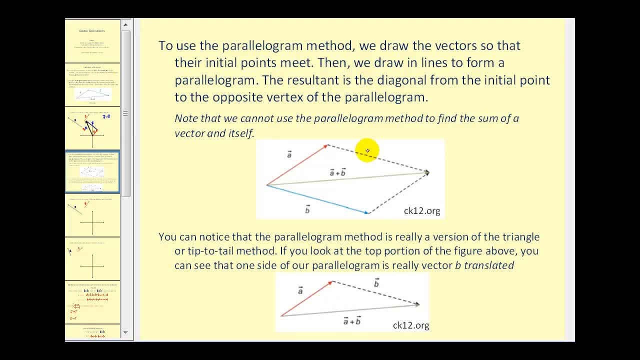 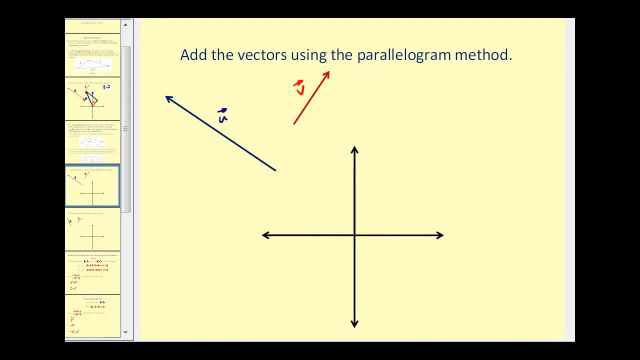 If you look at the top portion of the figure above, you can see that one side of the parallelogram is really vector B translated. Let's go ahead and add these vectors using the triangular method, So we'll place both initial points at the origin. Now we'll form a parallelogram. 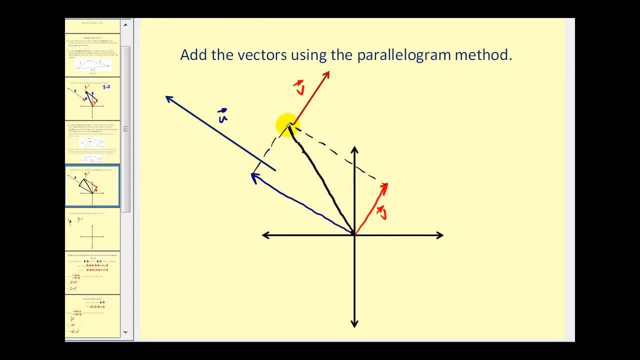 And the diagonal of this parallelogram is the resultant like: so: So this vector here is vector V plus vector U. Now let's go ahead and take a look at subtraction just for a moment. Notice on this problem: we want to have two times vector U minus vector V. Well, 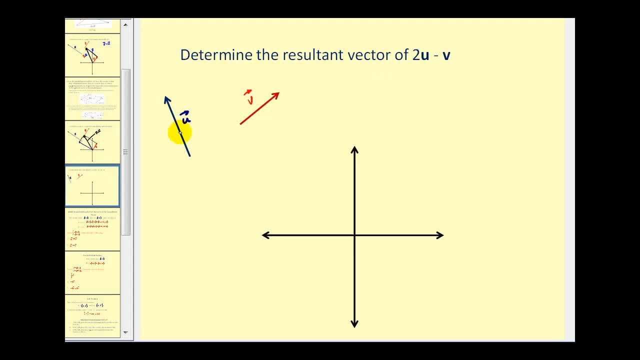 two times vector U means we're going to sketch this as a position vector, but we'll double the magnitude or double the length. So if this is U, this would be two U minus vector V. Now, because we're subtracting V, we'll actually graph V not in this direction, but 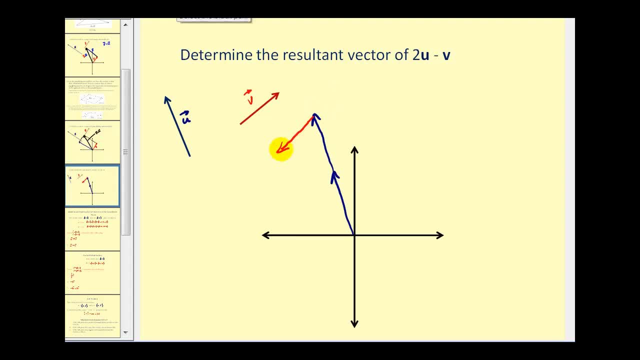 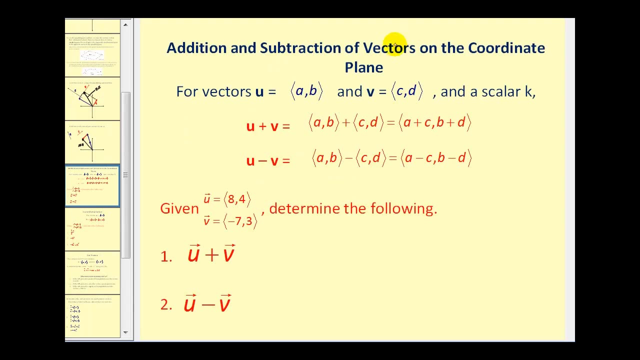 in the opposite direction, like so. So the resultant using the triangular method would be the vector that starts at the origin and has its terminal point here, Two times vector U minus vector V. Now, the addition and subtraction of vectors in component form is actually very 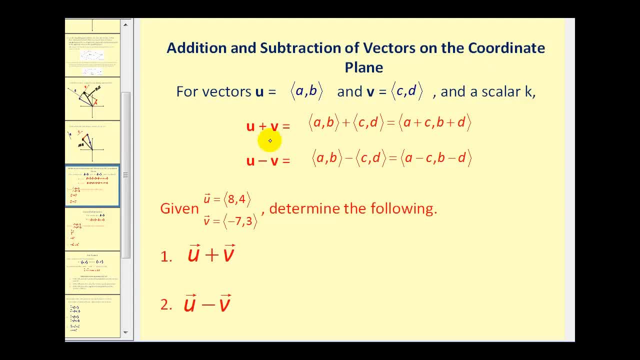 straightforward. You can see what we have to do to add to vector U. We have to add two vectors in component form is just add the horizontal components and add the vertical components, And for subtraction we just subtract the horizontal components and subtract the vertical components. If we have these two vectors and we want to find their sum, we 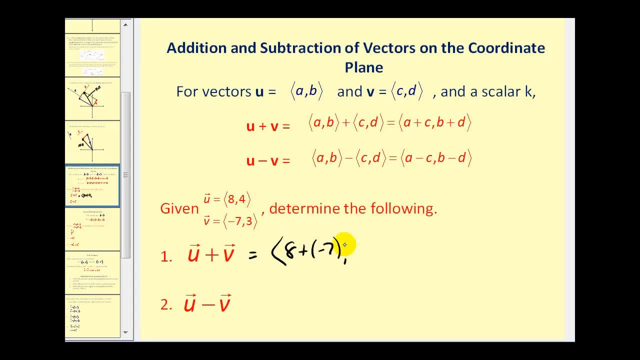 would have eight plus negative seven and four plus three. So we'd have the vector one: seven. So as you can see, it's very straightforward. And then for subtraction it's very similar, except now we just subtract. So I have eight minus negative seven and four minus three. 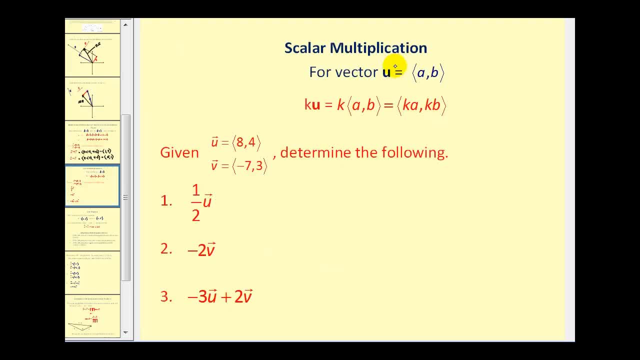 The vector fifteen one. Now let's take a look at scalar multiplication. It'll probably remind you of distribution. If you have K times the vector U, you just multiply each component by the scalar K. So one half times vector U is going to be one half times the vector. 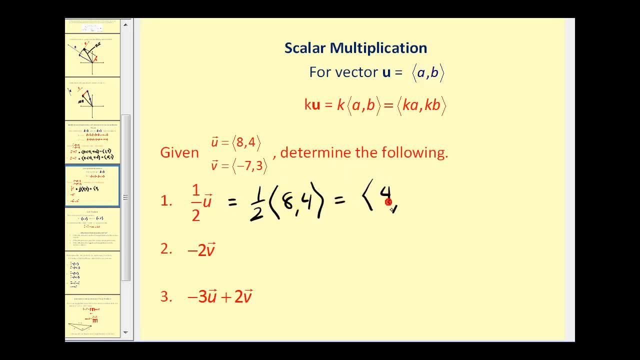 eight four. Well, one half times eight, four. one half times four, that would be two. So negative two times vector V, That would just be the vector with the horizontal component fourteen and the vertical component negative six. If we wanted to find the sum of these, 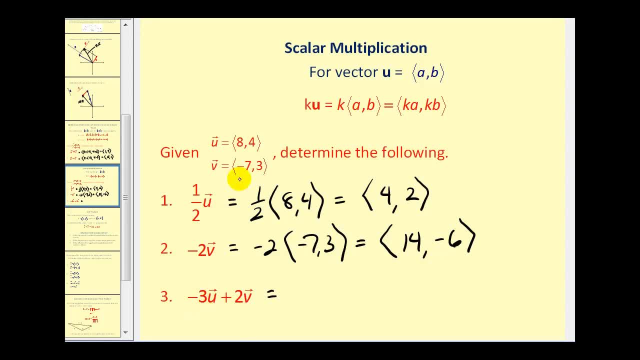 two vectors. we would first multiply vector U times negative three. Let's go ahead and do that first. Here's vector U, So we'd have negative twenty four, negative twelve. We want to add this vector to times vector V. That would be negative fourteen six. So the 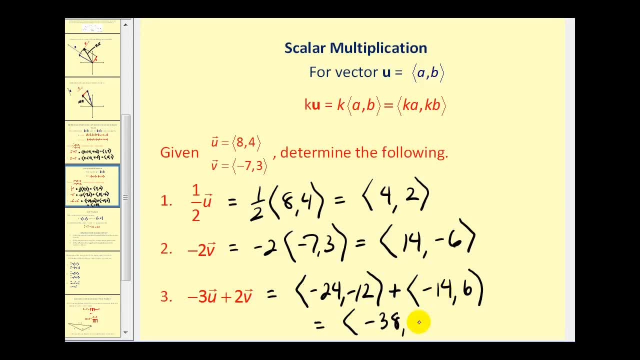 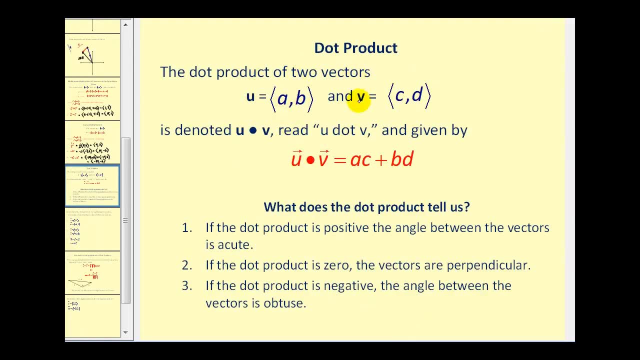 resultant would be negative thirty eight negative six. Let's finish off by talking about dot product. The dot product of vector U and vector V is denoted with this notation and it's read: U, dot V, And it's given by A times C plus. 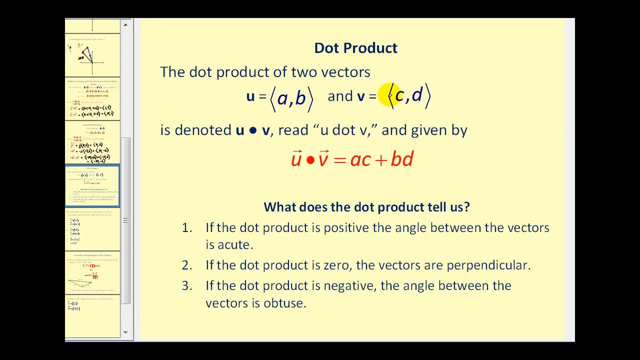 B times D. So we find the product of the horizontal and vertical components and then we sum them And the dot product does tell us some interesting information about the two vectors. If the dot product is positive, the angle between the two vectors is acute. If the dot product 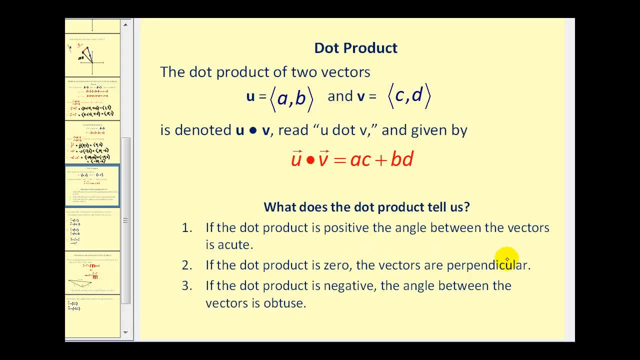 is equal to zero, the angle between the two vectors is acute. If the dot product is equal to zero, the vectors are perpendicular or orthogonal. If the dot product is negative, the angle between the two vectors is obtuse. Let's see if we can find the dot product for. 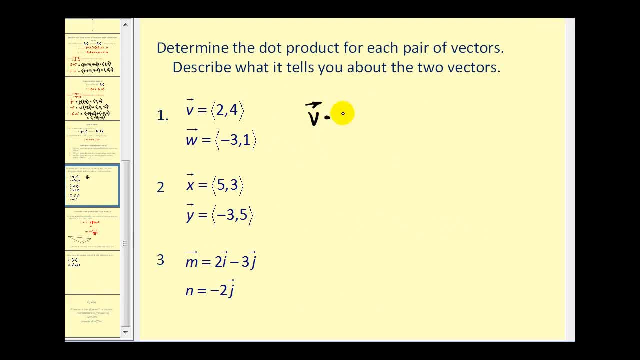 these vectors, V, dot, W, will equal two times negative three plus four times one. It would be negative six plus four negative two. Since the dot product is negative, the angle between these two vectors is negative. So the angle between the two vectors is equal to negative. 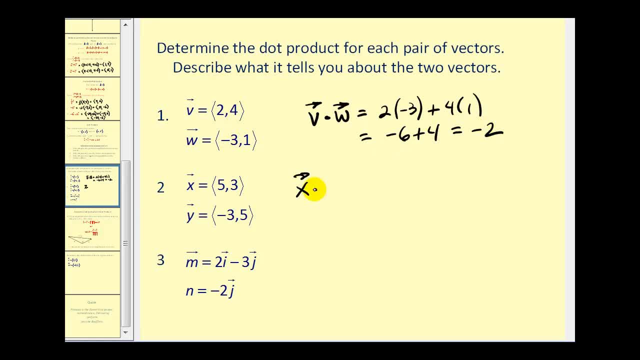 three plus four negative two. So the angle between the two vectors is an obtuse angle. X dotted with Y will equal five times negative three. that's negative. fifteen plus three times fifteen that's fifteen. that's equal to zero. So that means these two vectors are: 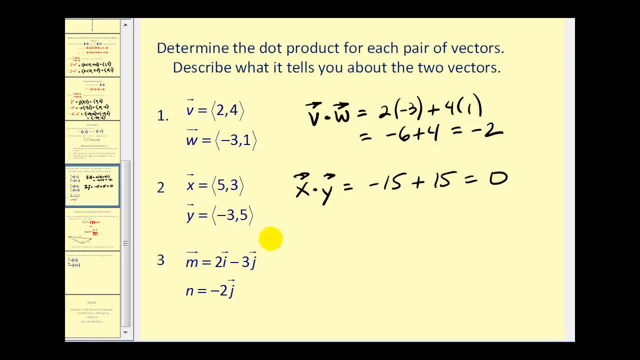 perpendicular or orthogonal. And then, lastly, we may want to rewrite these vectors in component form. This would be two negative three, and this would be zero negative two. So that's r. So that means the dot product would equal two times zero. of course that's zero plus. 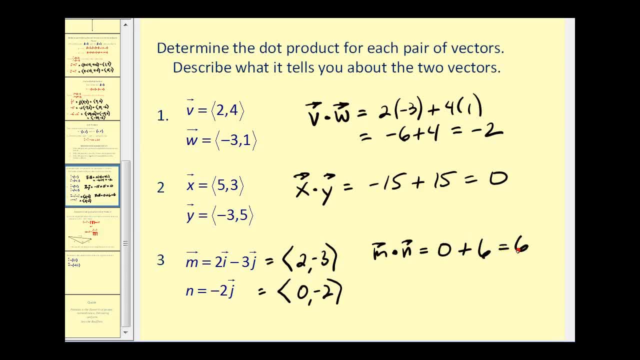 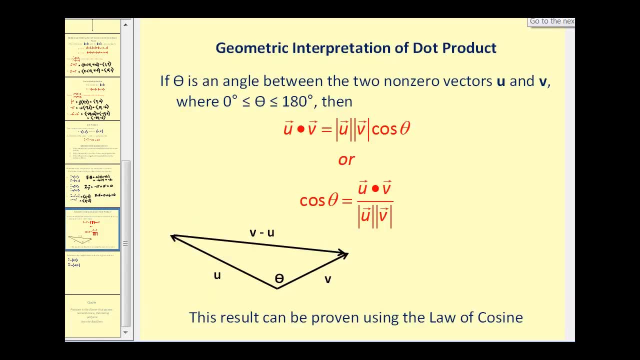 negative. three times negative two, that would be six. So now our dot product is positive. so the angle between these two vectors would be acute. Let's take a look at the geometric interpretation of the dot product. If theta is the angle between the two non-zero vectors. 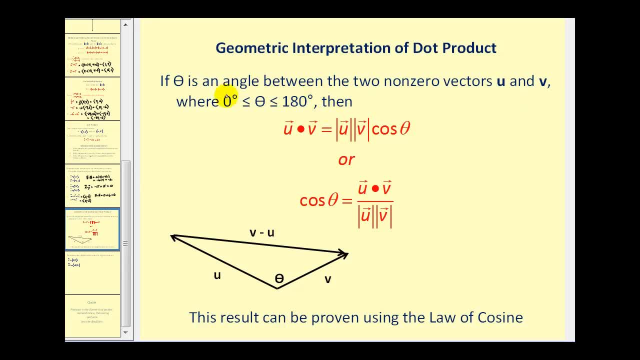 u and v. where theta is in the closed interval from zero to 180 degrees, then u dotted with v is equal to the magnitude of u times the magnitude of v times cosine theta. Or, if we solve this for cosine theta, we would have the equation in this form: 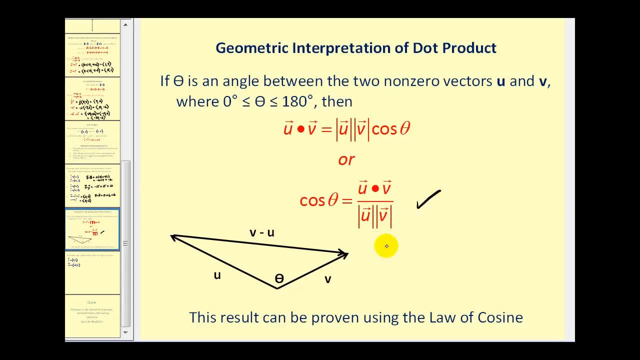 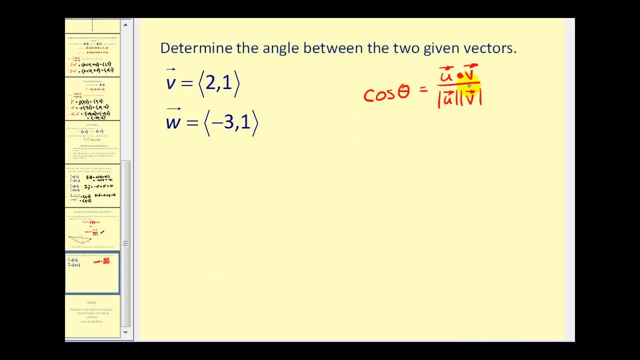 Now we can derive this formula by using a sketch similar to this and using the law of cosines, but right now we don't have time for that. Let's go and take a look at one problem. We want to determine the angle between these two vectors. 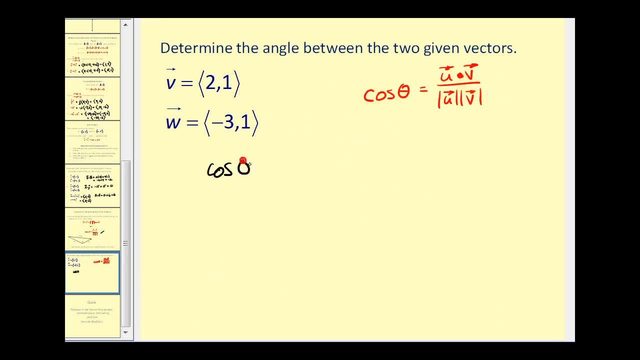 So, using this formula we're going to have cosine theta is equal to the dot product. So two times negative, three negative six plus one times one is one, All over the magnitude of u times the magnitude of v. Well, our vectors are v and w, but it's the same idea.